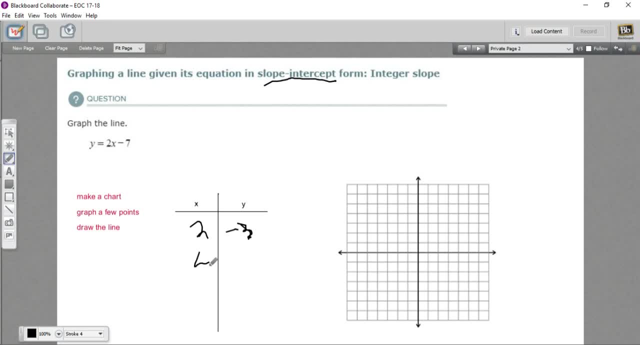 All right, and let's put in another value here. Let's put in 4.. So 2 times 4 is 8, minus 7 is a positive 1.. Let's just do one more. So 2 times 5 is 10, minus 7 would be 3.. 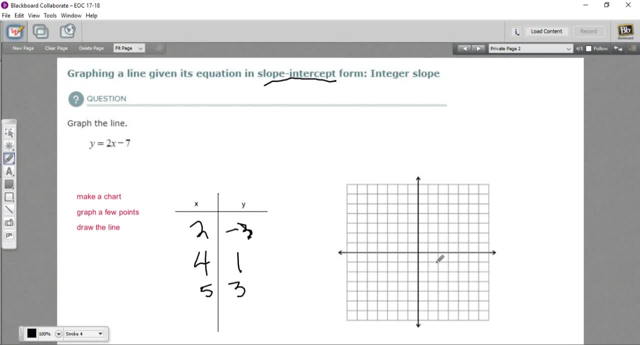 So now we've got three points. We can really double check our work here. Let's plot these: 2 on the x is negative, 3 on the y and 4 on the x is 1, and then 5 on the x is 3.. 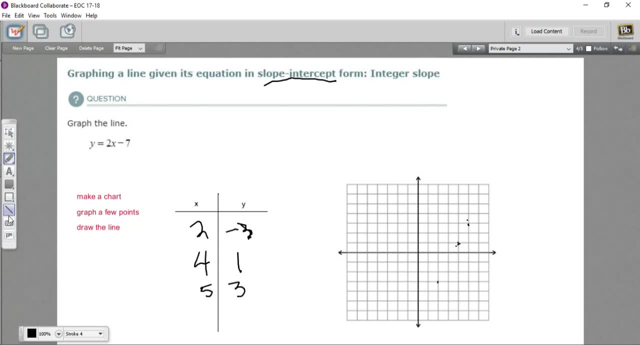 All right, so it looks like they're all lining up. We can draw the line in now. All right, so there is our line. y equals 2x minus 7.. I just chose some values for x and I did the math here. I multiplied them by 2 and I subtracted 7 to find the y. So that's one way. 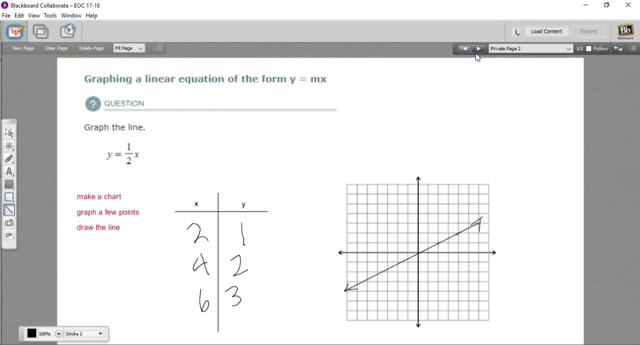 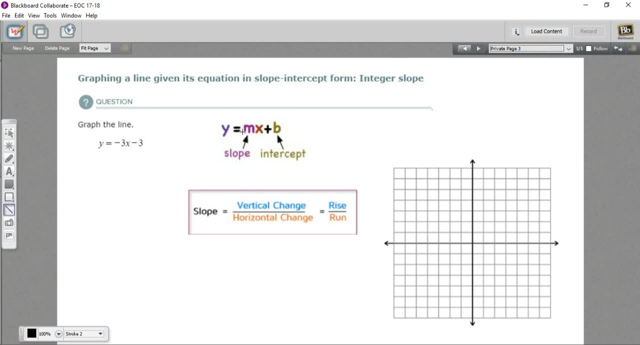 to handle these. There is another way and you might think of it as a shortcut. Whoops, there we go. So I mentioned this is called slope intercept form. In this form, whatever number here is multiplied by the x is the slope, and whatever number comes after that that's not multiplied by the x is what we 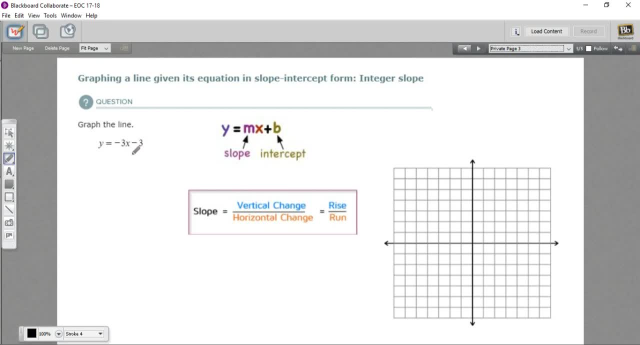 call the y-intercept. In this case, we have a negative 3 for our y-intercept. What that means is, on the y-axis, this line will cross at the point negative 3, where y equals negative 3.. So we've got one point already just by looking at the equation. 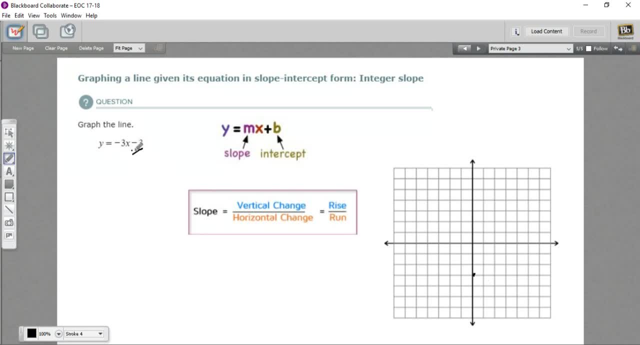 And then you can get another point or two just by applying the slope. and for this we have to understand what slope is: The number that's multiplied by x. that's our slope. In this case it's a negative 3. And what we want to do is think of slope as a fraction of the vertical change over. 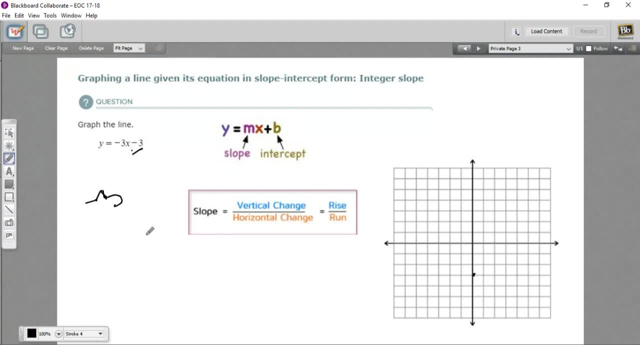 the horizontal change or the rise over the run. but negative 3 is not a fraction. Well, luckily for us, we can write any number as a fraction by just putting it over 1.. So this is negative 3 over 1.. So this is our y-intercept. 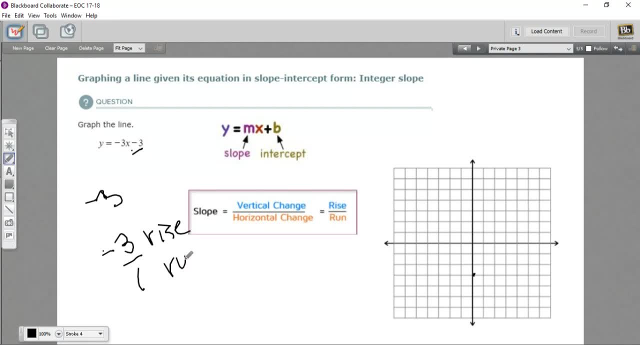 rise here and this is our run. what rise mean means is how many spaces it goes up, and what run means is how many spaces it goes over to the right. we've got a negative number for rise, so that means it goes up a negative three, which is: